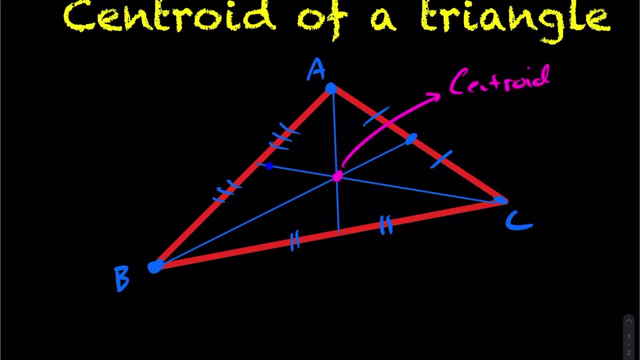 But to calculate the centroid you don't have to intersect all three median lines to find the answer, You only just have to intersect two. So to find the centroid of a triangle, the only thing you have to do is find the point of intersection of its median lines. 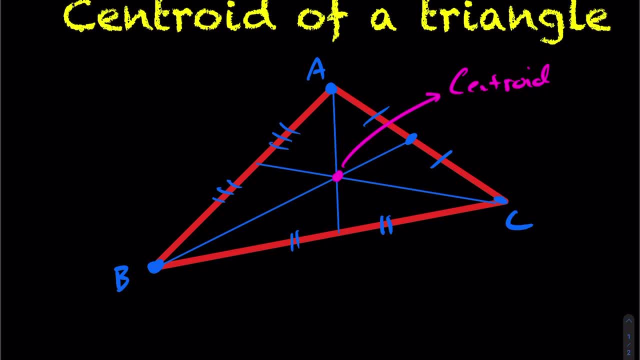 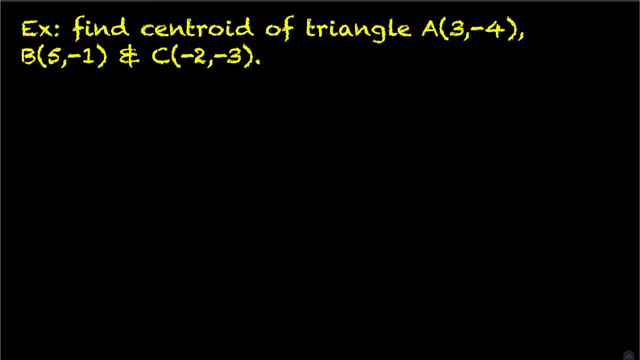 Since all three median lines intersect at the exact same value, you only really have to find the intersection of any two median lines. Okay, let's take a look at an example of calculating the centroid. So if we want to calculate the centroid of this triangle here, 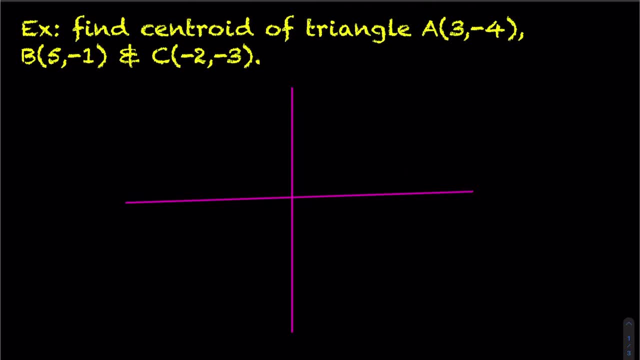 you can do a rough sketch as to where the centroid is. So if we want to calculate the centroid of this triangle here, you can do a rough sketch as to where the points are. Again, we've been talking about this for some time now. 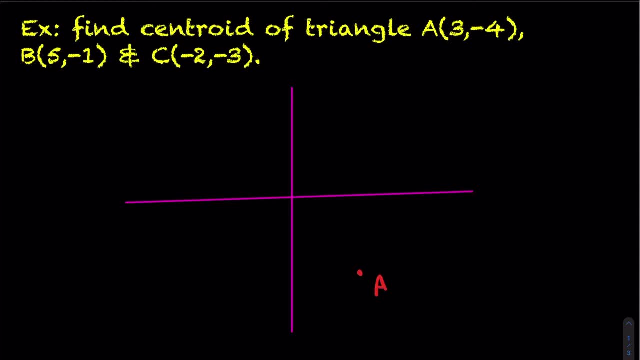 It just gives you an idea of where everything's at. So we've got the point A: 3, negative 4.. The point B is 5, negative 1.. And then the point C is going to be negative: 2, negative 3.. 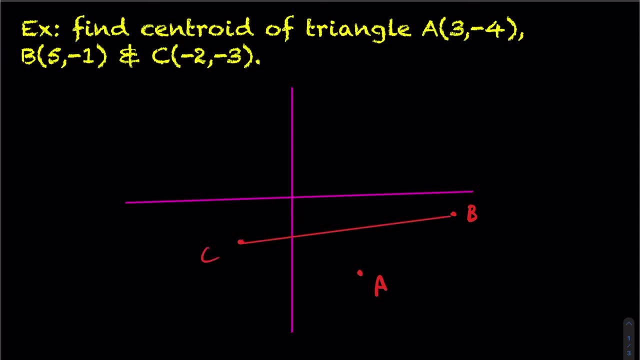 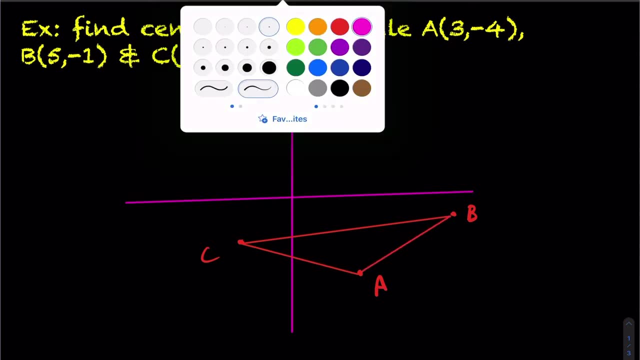 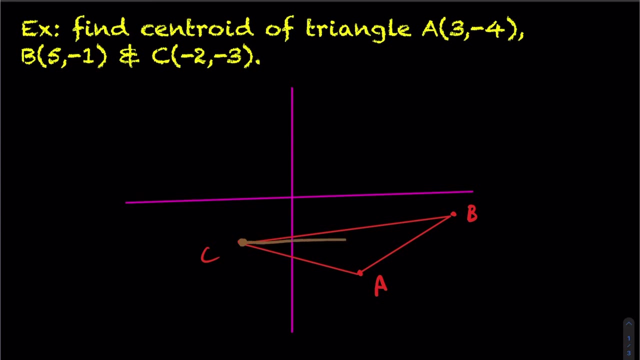 So we have our point C here. So a rough sketch of this triangle would look like this. Now, if I want to go ahead and calculate the centroid of this triangle, what it is by definition, as we talked about, it's the intersection of two of the median lines. 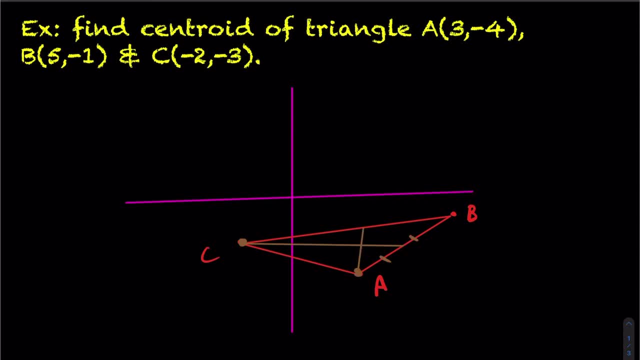 So maybe we've got a median line here and then maybe the other median lines right here- All right, and we would have to find the point of intersection of these. So the long way of doing this is to actually calculate this equation. calculate this equation, then find the point of intersection of them. 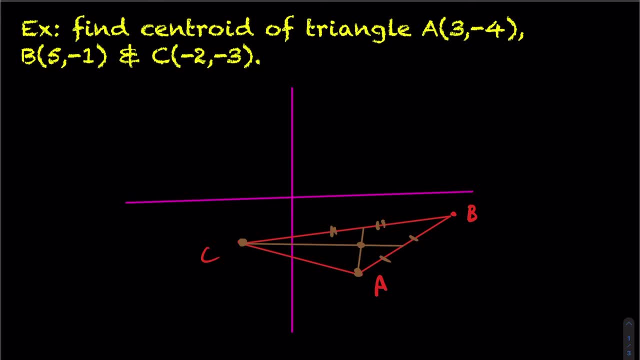 And that point of intersection would be your centroid. There is a quicker way. So the quicker way is since you're balancing the weight of the object out. if I want to calculate, If I want to calculate the centroid of a triangle, the only thing I have to do is add up all of my x's and average them out. 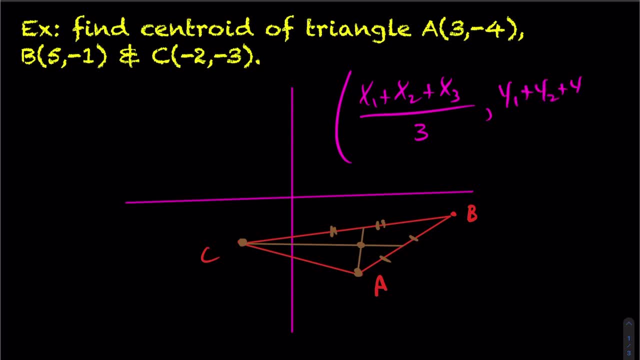 so divide by 3,, add up all of my y coordinates, add those up, divide by 3, and you're done. This is all you have to do to calculate the centroid of a triangle. Average out your x's, average out your y's. 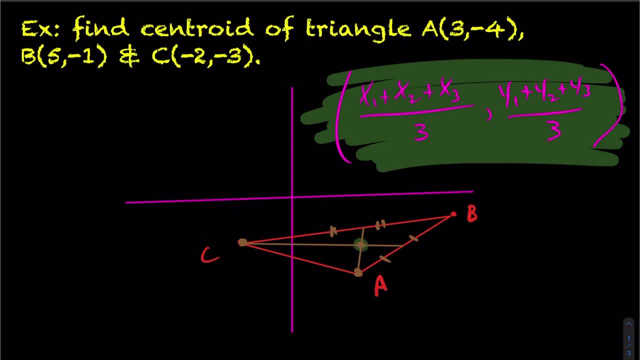 you'll average the weight of the object out, finding your centroid. So if I want to go ahead and calculate the centroid of this triangle, to calculate the centroid of triangle a, b, c, the only thing that I have to do is add up my x's.